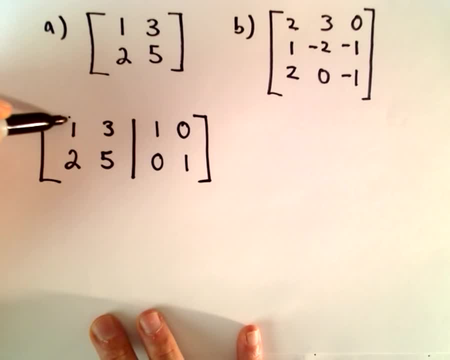 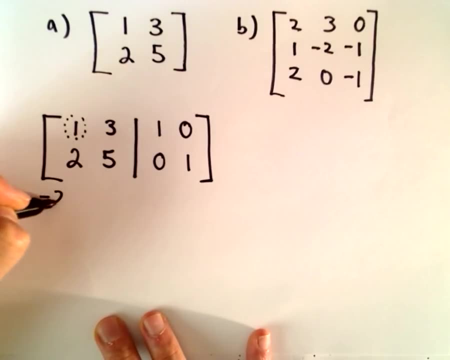 Well, I've already got the 1 in the top left entry, which I want to have, So I'm going to get a zero below it. So to do that, I'm going to take negative 2 times the first row. Add that to my second row. 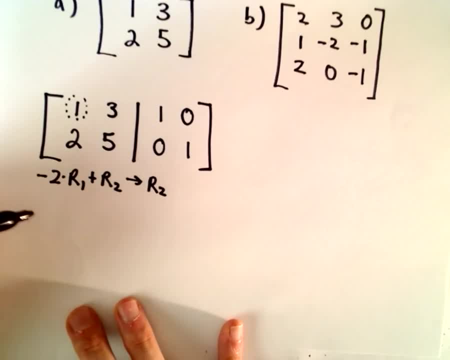 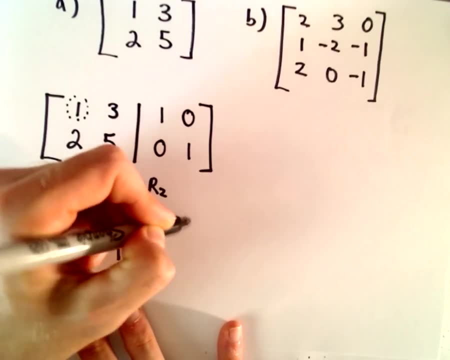 And that's going to become my new row 2.. So if we do that, okay, the first row we just leave it alone. Leave it alone. I almost messed it up already. So there's my bad-looking 1 there. 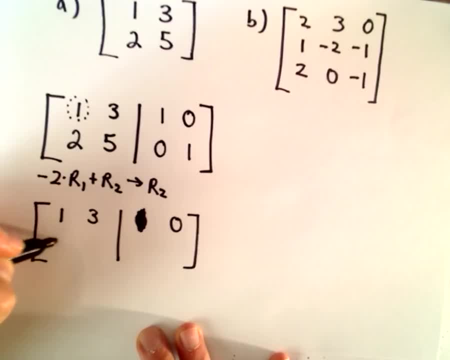 So if we do negative 2 times 1, that's negative 2. Negative 2 plus 2 will be 0. Negative. 2 times 3 will be negative 6. Negative 6 plus 5 will be negative 1.. 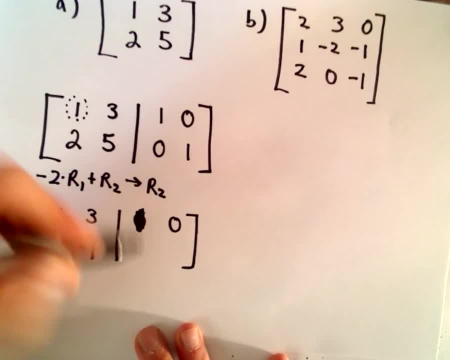 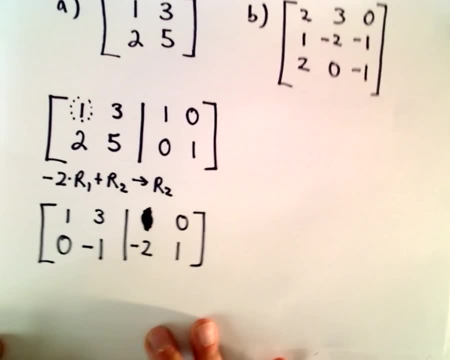 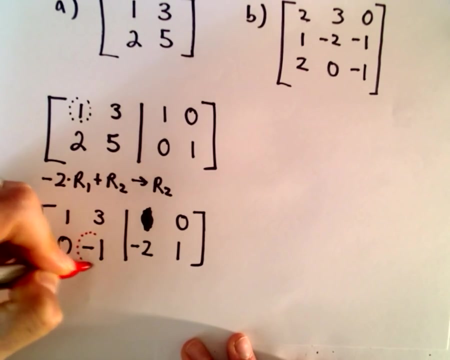 Negative 2 times 1 is negative 2.. Plus 0 will be negative 2. And then negative 2 times 0 plus 1 will just be positive 1. So that one not too bad at all. So now again, we just want to get this entry with a negative 1.. 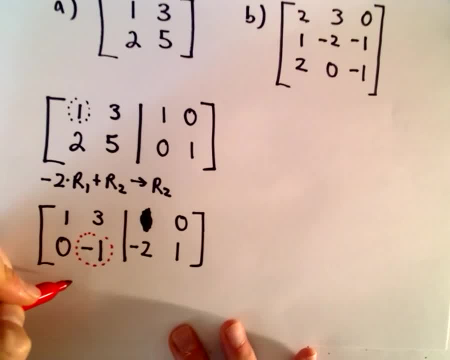 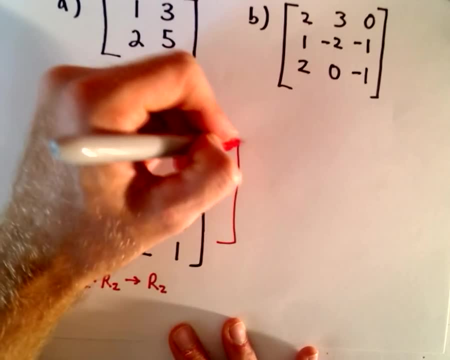 We want that to be a positive 1.. So all I'm going to do in that case is I'm just going to take negative 1 and multiply that by row 2 to get my new row 2.. So we'll put that right up here. 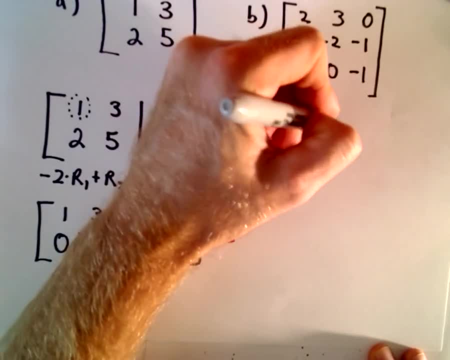 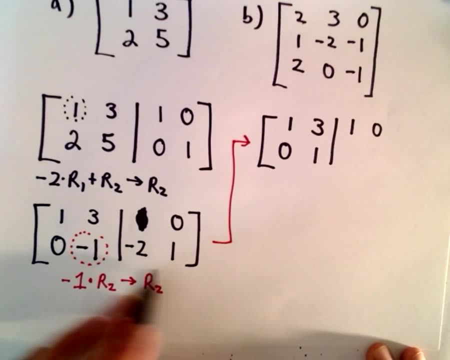 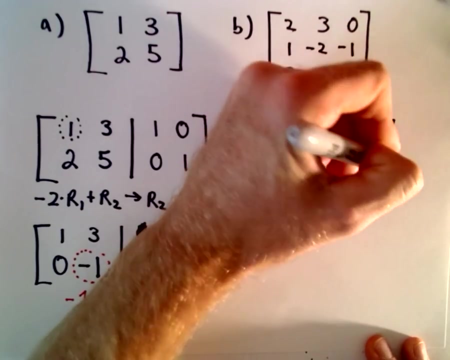 So again, not much to do in this step. The first example here, trying to give one that's not super terrible. So all that's going to do is it's just going to change the signs on the second row. So I have positive 1, positive 2, and negative 1.. 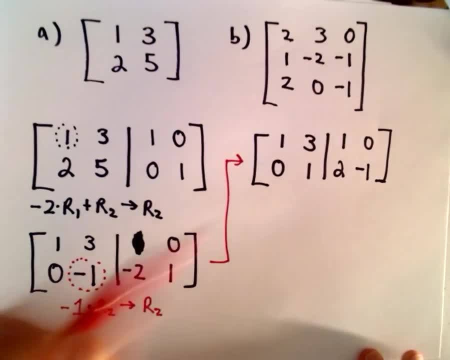 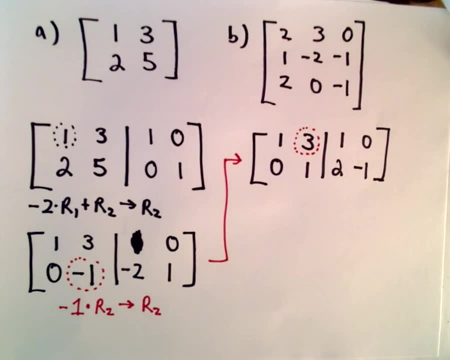 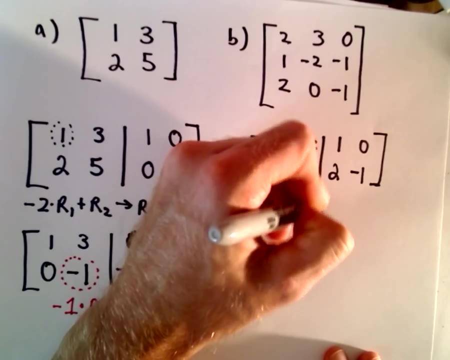 All right. so now all I want to do is I want to make this entry where we have a positive 3, I want that to be a 0. And then we'll have the identity matrix on the left side. So I'm going to take negative 3, multiply that by row 2, add that to row 1 to give me my new row 1.. 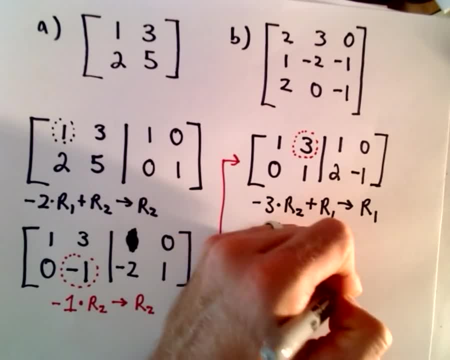 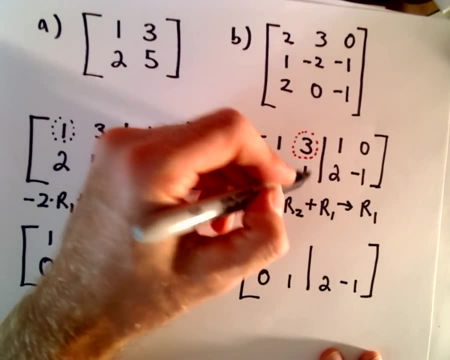 So I'm going to go ahead and write down the second row, since I'm not changing it. Okay, so negative 3 times 0 plus 1 is 1.. Negative 3 times 1 plus 3 will give us 0..